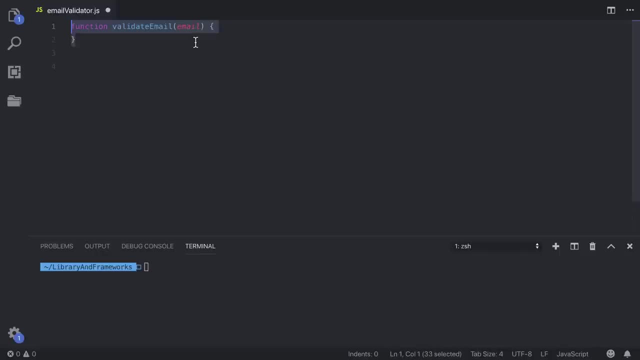 So let's take a look at an example where we actually use a library. So let's take a look at an example where we actually use a library. So let's take a look at an example where we actually use a library. So we actually wrote a function that validates email earlier. So we're going to write a function called 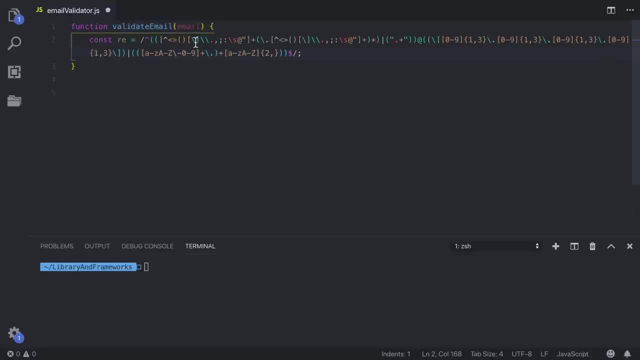 validateEmail. that will take a parameter called email And from there we're going to write our regular expression And you can see it's quite lengthy and tedious and it's hard to understand If you're not familiar with regular expressions. they basically match a string with specific. 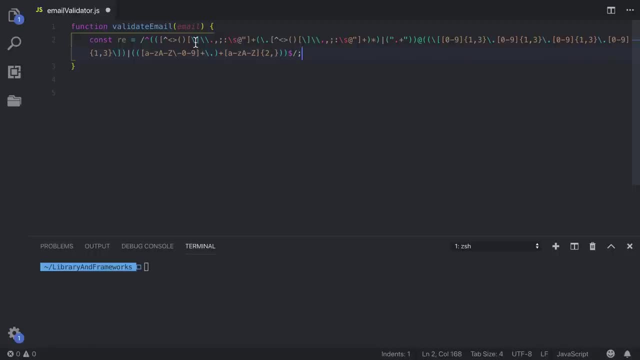 characters And this is basically a pattern that actually looks for the specific email that matches the pattern. So near the end of the function we're actually going to return a Boolean that will check whether the email has passed a read regular expression test and it 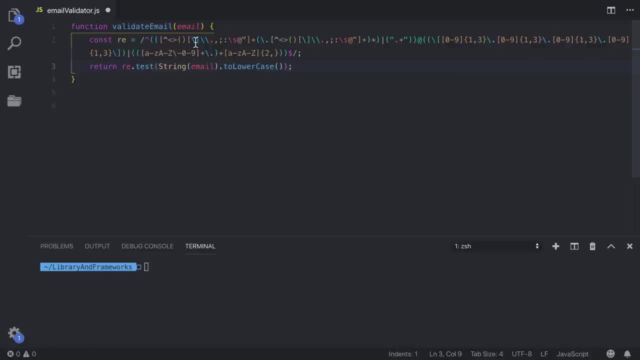 will tell us whether the email was false, which was in, which means invalid, or true, which means that it was valid. so let's actually go ahead and test this out before we start. let's go ahead and validate an email that has the wrong characters, so I'll pass in a string that simply says name comm, save that and then. 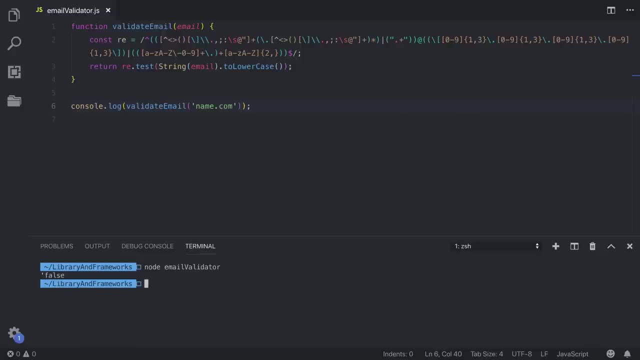 we're gonna run the validator and you can see that's false. I put a little quote there accidentally. I'll run that again and you can see that's false. so if I type in an at gmailcom and save that, that should return true. so the regular. 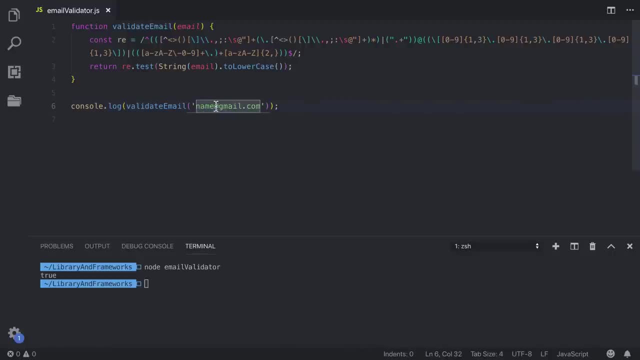 expression is essentially looking that there's characters and it's split by an at sign and it has another domain name here, followed by a period and then another three string character or a specific number of characters here. now all those. this works totally fine and it's acceptable code. there's nothing. 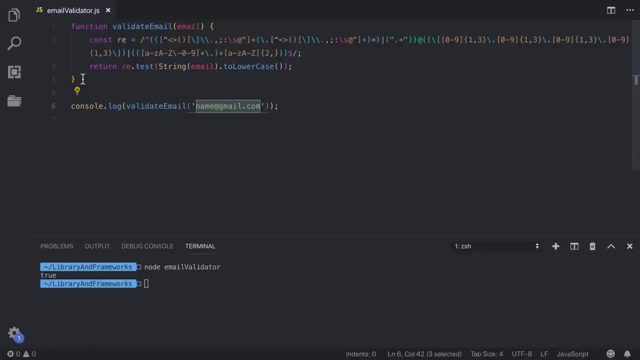 wrong with it. there's a faster way to do this by using a library called email validator. now, email validator essentially has this function, kind of similar to this, but it goes in a lot more depth as to what are valid emails or not. here it's probably not testing. 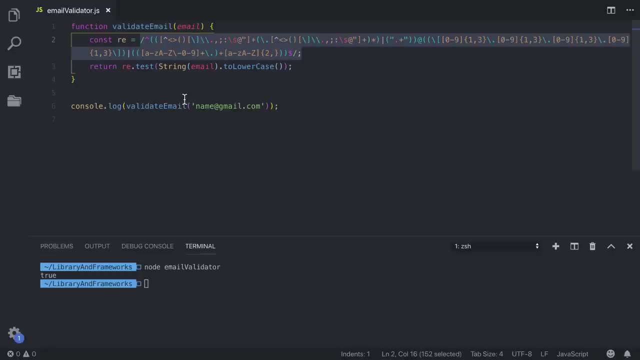 all the cases for specific emails, but the specific library email validator can check for a bunch of different emails with different domain names, different lengths, different symbols and many other ways of writing an email. so I'm gonna go ahead and move this down and import that library and you'll see how. 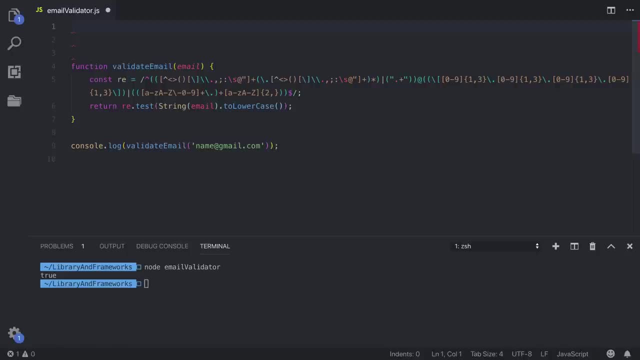 much more succinct and condensed. our code looks. our code looks using this library. so I'll import the library at the top here and I'm gonna call it validator and we're gonna require it into this file. now the library name is called email validator. and now what we do now that we have validator- the 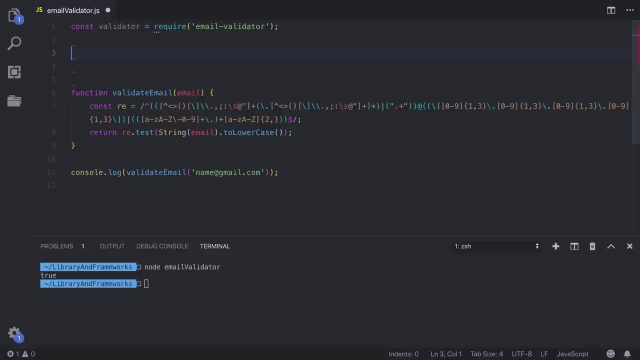 library itself. we can call a lot of their methods that are actually written in that library using a period. so we can simply type in: well, console lock this as well, validator dot- validate, and then here we type in the name, the email that we want to check. so I'll do the same with that we did. 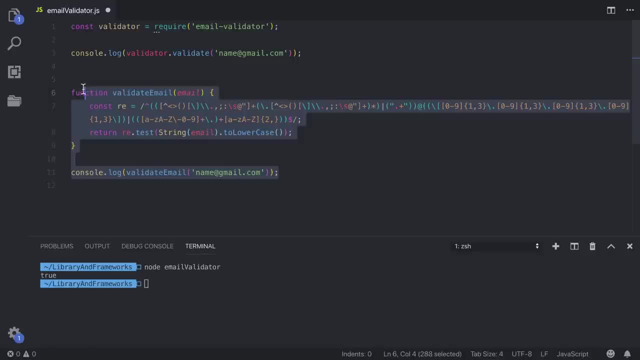 earlier now. I'm actually gonna comment this out so we know we don't get confused here. I'm gonna save this and clear this console out again and we can see that it's actually true. so let's say, let's remove the at sign to make sure. 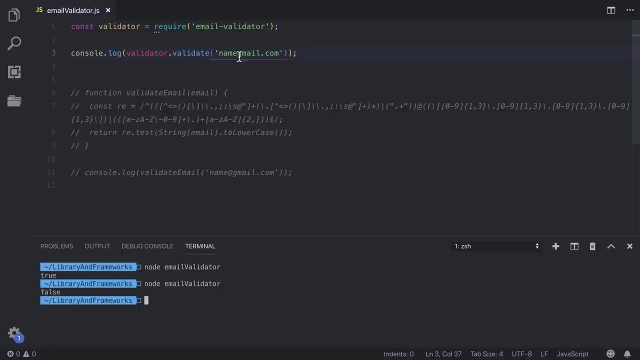 that it's invalid and we see now we get a false. so you can see now how a lot more of the code is being written in here. so if we want to condense, our validator is simply importing. the library allows us to reuse this kind of function into this. 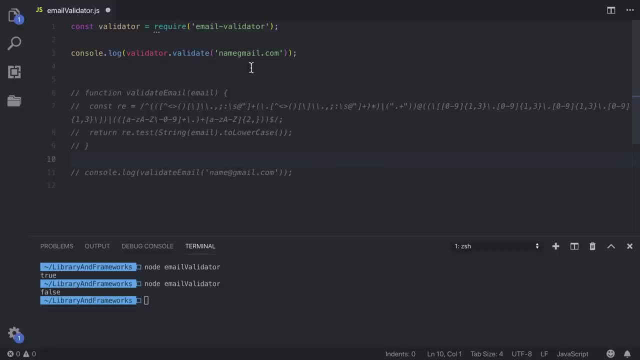 file and really condense it and make it really readable and easy to to use. so let's say we have this validator when signing up a user, but we also want to validate users when logging in, so we can simply import this library on the login page and do the exact same thing we've done here, instead of actually running a. 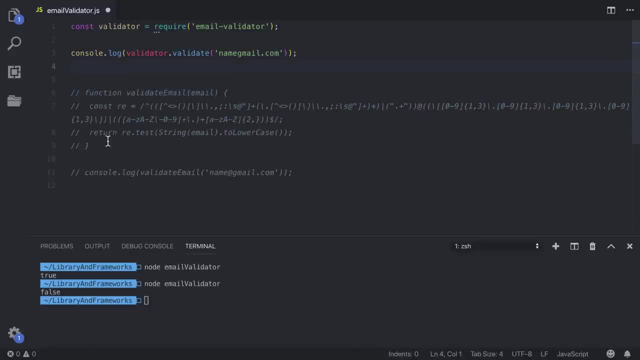 long, tedious function using regular expressions like the one below. so we can see that we're actually using this handy function from the library instead of writing this function over and over again in different files. now, in theory, you could actually write this function in a utilities file of your own project. 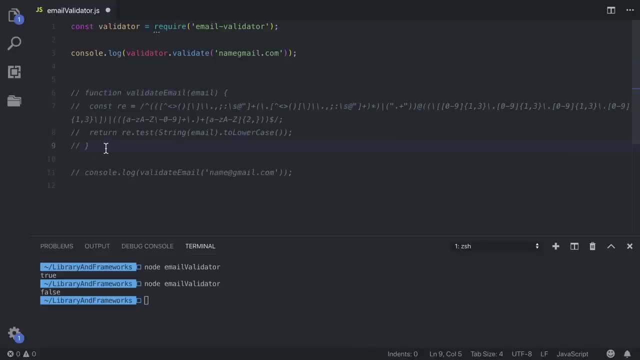 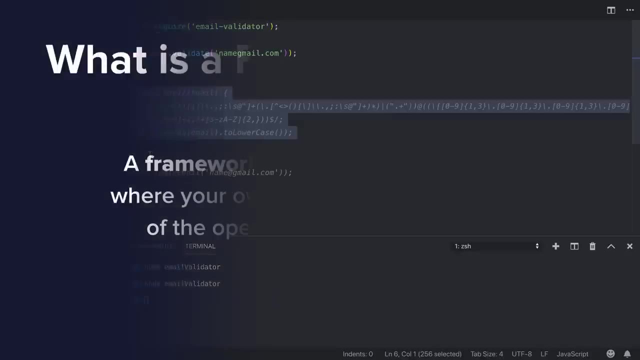 and save it there and import it in other files, but you're essentially running a library on your own and since there's already an library for email validation, you might as well just use the one that's available. now let's take a look at what is a framework, and it- just a framework- is a supporting structure. 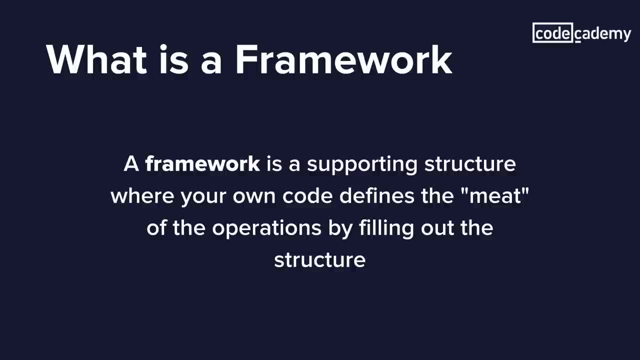 where your own code defines the meat of the operations. by filling out the code, it essentially provides a scaffold on which to build software and allows a programmer to avoid writing any boilerplate code and merely fill in the blanks, leaving the framework to decide when it's appropriate to execute any 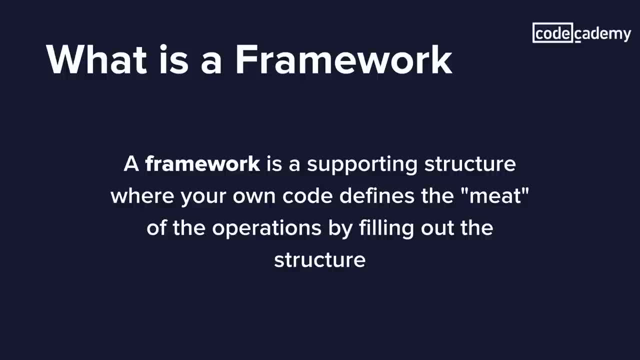 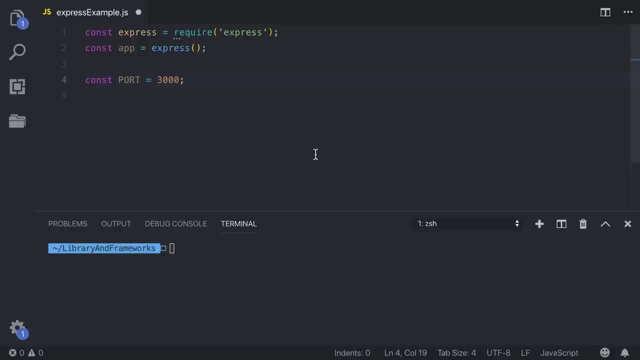 business logic. so let's go ahead and take a look at an example of how we would use a framework. we're gonna be working with one called Express now. Express is a framework that provides a robust set of features for web and mobile applications. now, I'm not going to go too in-depth as to what Express is. 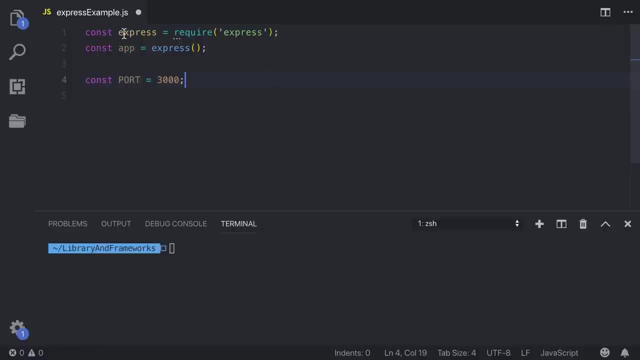 since this isn't really a tutorial on it, but I do have some boilerplate code here where I'm actually importing the framework at the top, I'm making an instance of the application itself and sending it to a variable called app and I have a variable called port, set to the number 3000, which we're going to be. 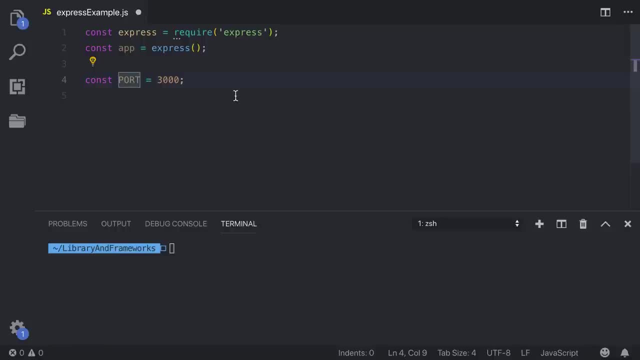 using in a second. now, when using Express and similar to other frameworks, it's structured in a specific way where it's going to be looking for specific method calls and specific parameters. so when you're actually using Express and you have to be able to name them- the methods correctly, you can just name them. 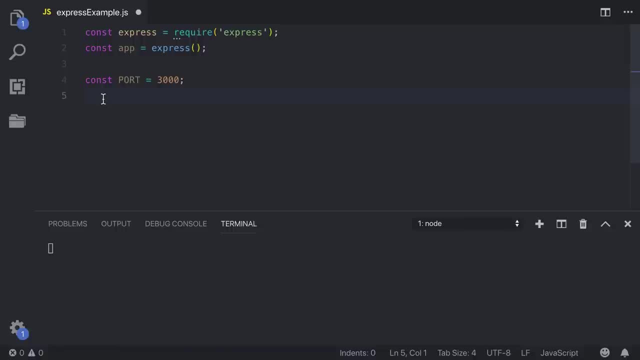 whatever you want. so let's say we want to make an actual get request on our root path and we already have an actual Express server instantiated and stored in our variable called app. now app will have a bunch of methods that is expecting, and one of them is actually dot get. so dot get is basically saying: 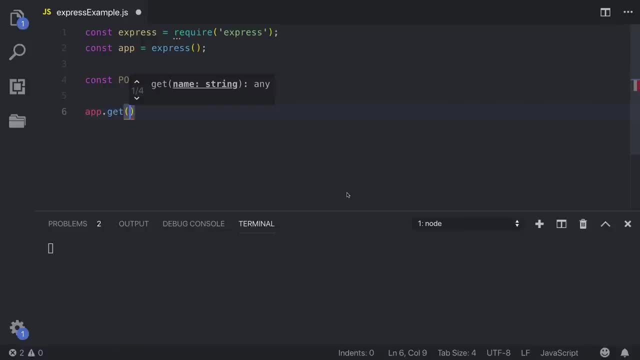 that when it gets to that route, it should give the response that is specified in the function, and it will take two arguments. the first one will be the route path, which will be our route path, which is simply a forward slash, and then it will take a callback function that tells Express what to send back to. 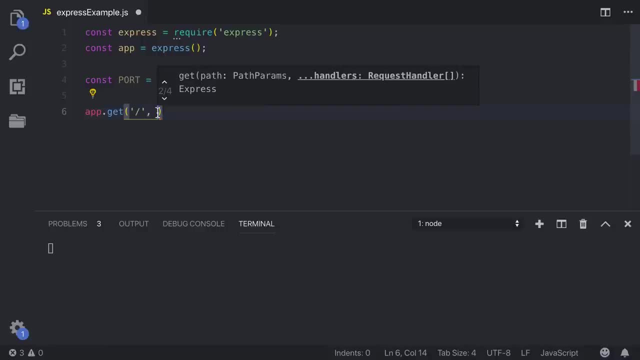 the person making the request. now, that callback function will take in two parameters as well- request and response- and these are essentially objects that Express knows how to handle and manage, and it's essentially going to be looking for them when this route is hit. so what we want to do is simply send a message. 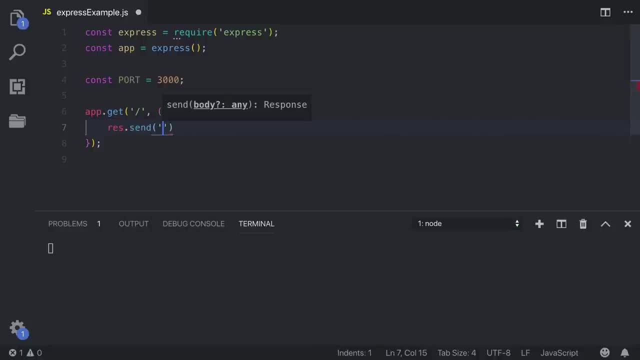 to the route and let's just send back a message that says hello from Codecademy. just like our app instantiation, our response object has also a bunch of functions and methods, that is, are available and we can invoke them whenever we want. so before we actually run this, we actually have to instantiate. 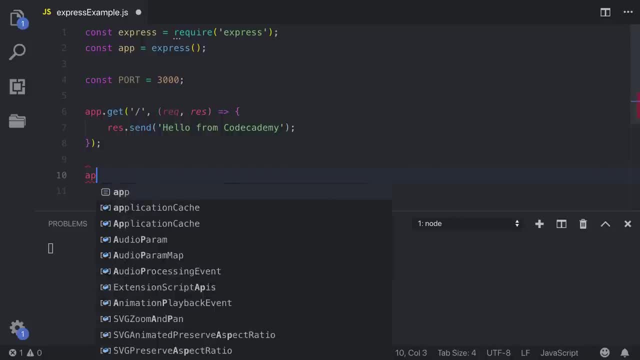 our server as well, and we can do this by simply calling dot listen and passing in our port. we start my server here and then we could simply let me save this and then let's go ahead and run our server. so I have a new tab open and I have set up my 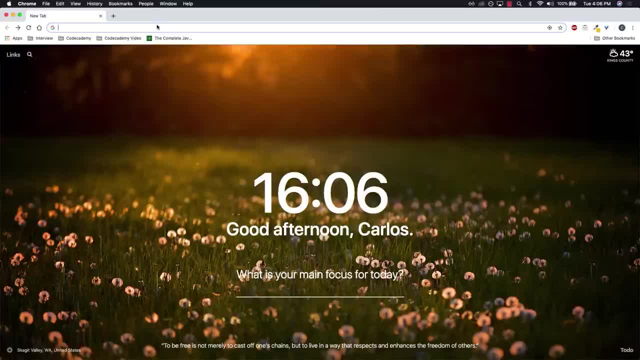 port on 3000 so we can go directly to our localhost 3000 and whatever we have sent through the dot send method call the string that we passed in there in the response object should display to the client here. so let's go ahead and go. 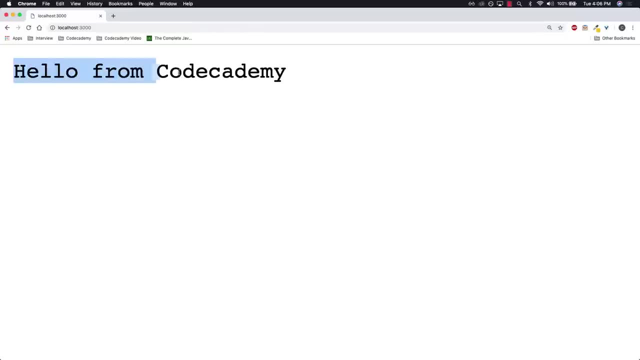 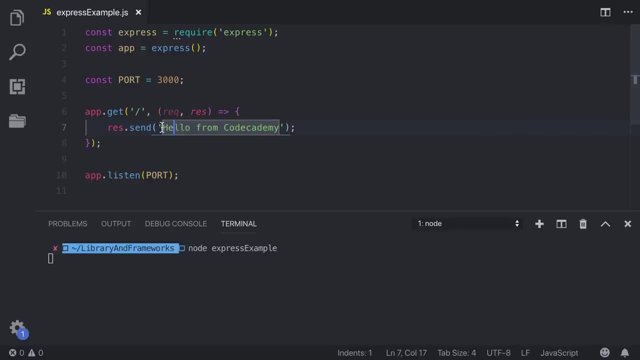 to our localhost 3000.. and you can see that the string that we passed into that function call is sent back to the user, to the client. So that's what was written right over here. So it's okay if you don't completely understand. 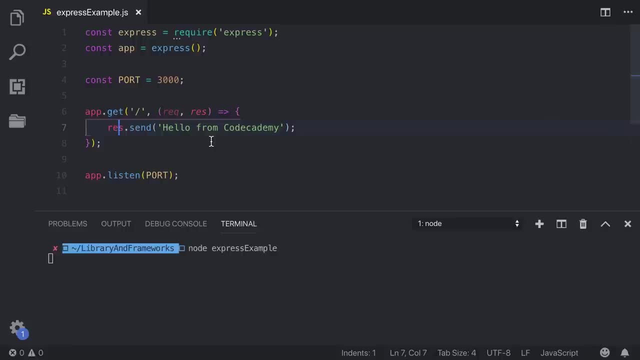 what the code means in here. Like I said, this isn't really an express tutorial, but what I do want you to get out of this is mostly how we're actually working with a framework, as opposed to a library where we simply import it. 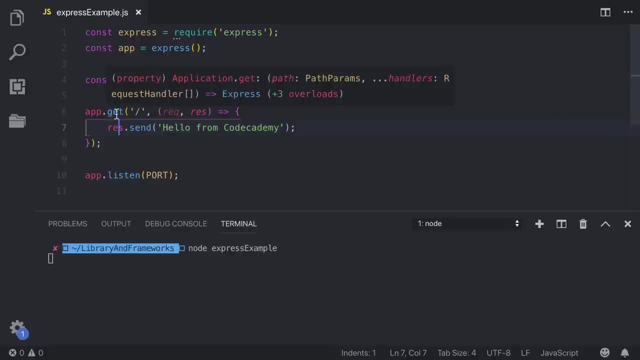 and call a method or a different method with different parameters. In this case, there's a specific structure that we have to follow. So if we're making a GET request or a POST request, it's gonna be expecting two parameters at least, one of them being the route. 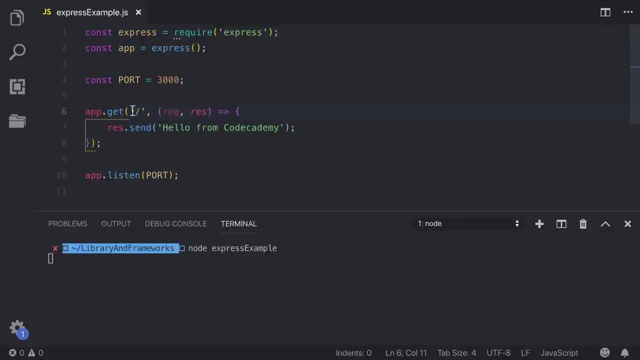 and the other one being a callback function. So if one is missing or the certain pattern here is like not a string, it's gonna give you errors. So you have to follow the pattern and the structure that the framework provides. So in this case, 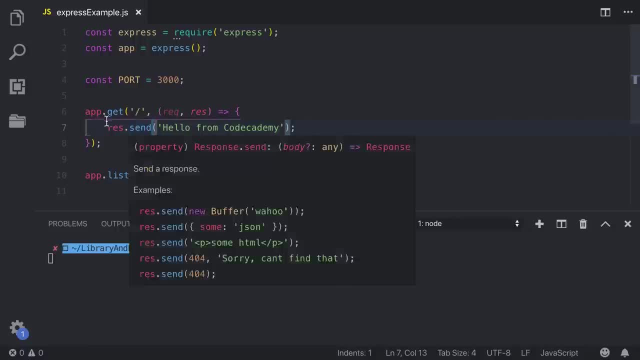 we're more of filling in the functions themselves instead of making simply method invocations, like we're doing with the library. In this case, the framework is calling on your code, You're not calling on the framework's code. So let's take a look at an analogy. 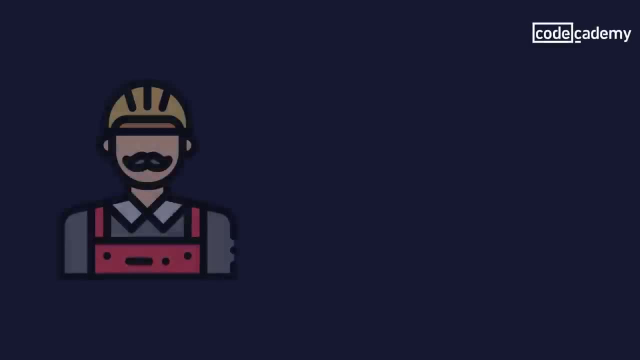 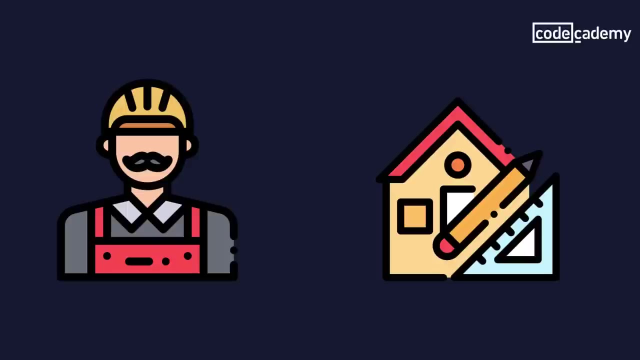 in order to drive this home. Let's pretend you're a construction worker and you're assigned to build a house. Now, in theory, you could build a house without using any tools, but if you wanna make your life easier, you'd go ahead and use a hammer, use a nail gun. 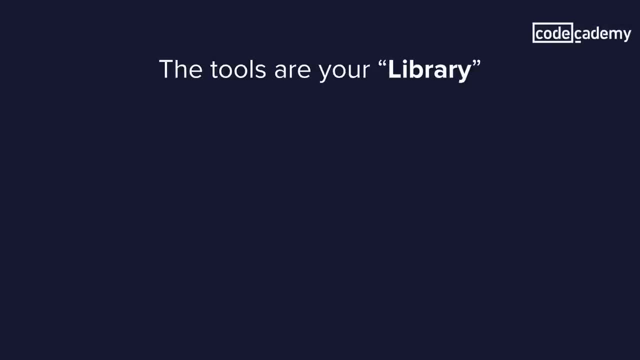 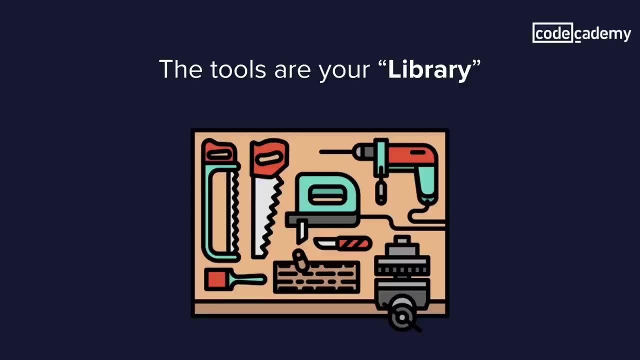 use a handsaw, whatever you'd need. So, in a sense, all these tools are your library. You're gonna be using these tools to build a house, and not only can you build a house with them, you can go ahead and build a table, a chair. 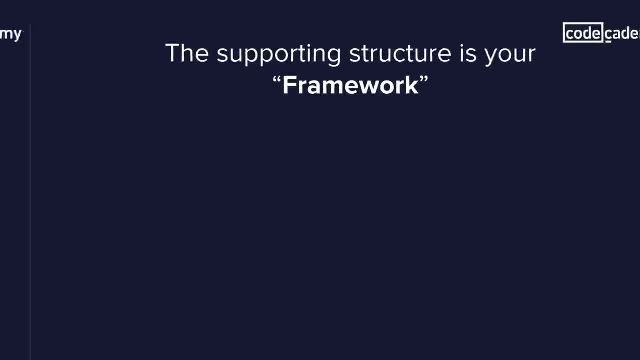 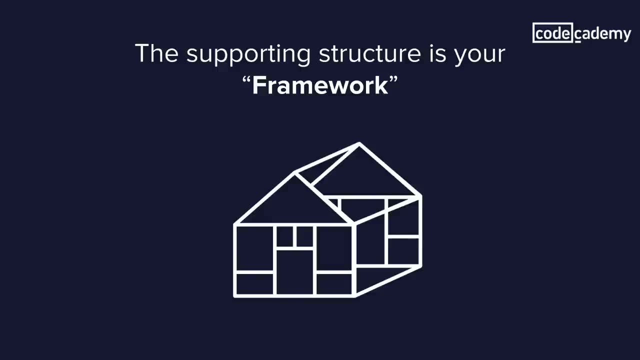 anything you like with these tools. Now, if you look at a framework, well, the supporting structure is gonna be the framework itself, So the framework dictates how your project will be structured, whereas libraries are more of the building blocks that can be used anywhere. 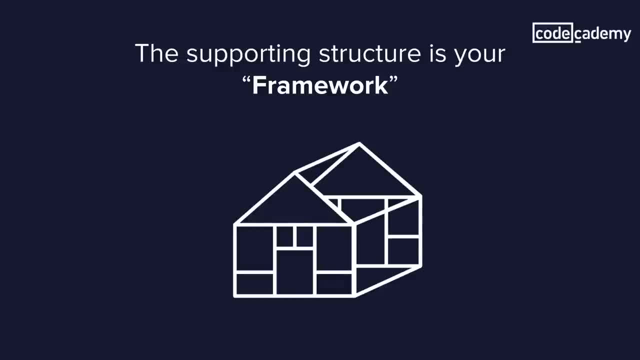 So the skeleton or foundation of the house is essentially your framework. You're gonna be adding to it and we're gonna fill out the structure until it's completed and it comes together. Now, one key point to note here is that a framework may use libraries. 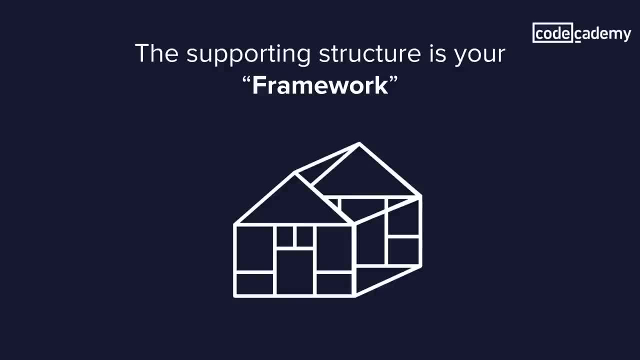 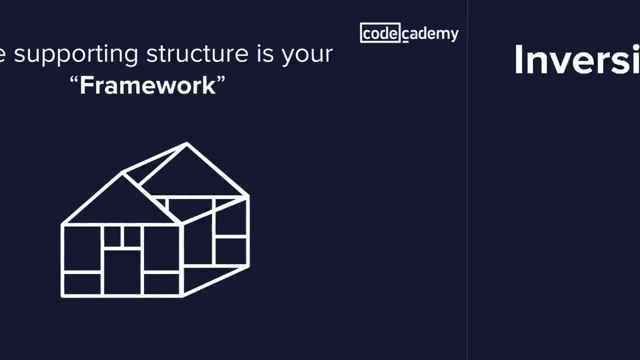 but it doesn't really need libraries in order to, I guess, in order to operate. So now we have an idea of what a framework and a library is, but one of the biggest factors that differentiate a library and a framework is something called inversion control. 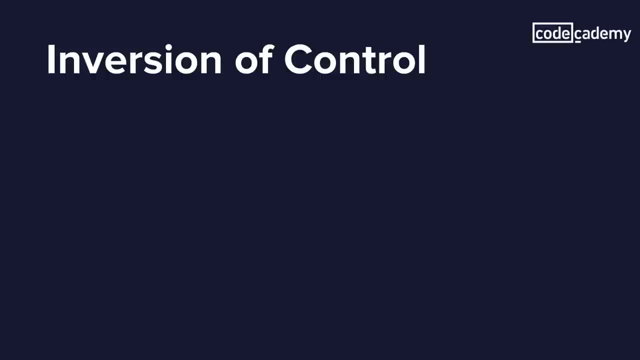 When we use frameworks and libraries, our code flows a little bit different. So let's say you have your own code written and you import a library. When you import a library, you have access to all these methods that are collected pieces of functionality from that library. 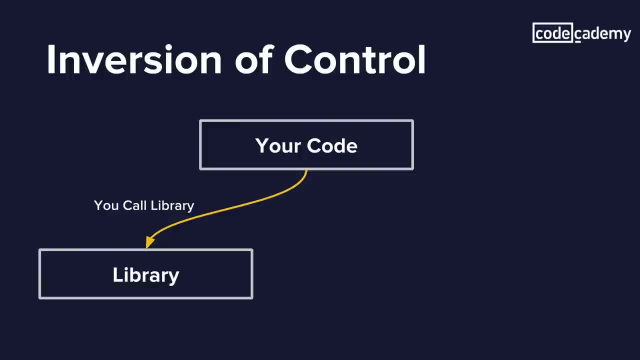 So you're making calls directly to the library itself. So when we use a library, we are in charge of the flow of the application. We are the ones choosing when and where to call the library. On the other hand, when we use a framework, 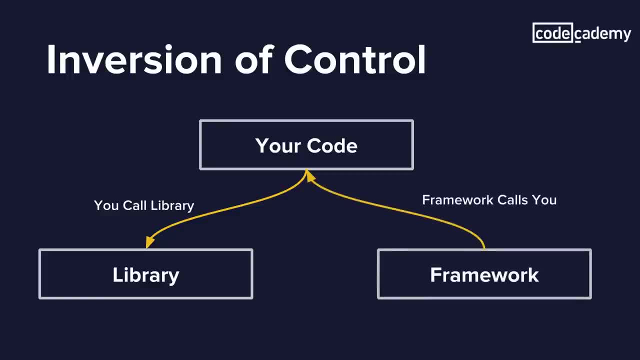 the framework itself is making calls towards our code. So the framework writer writes the application and leaves out the interesting details which we fill in. So when using a framework, the framework is in charge of the flow. It provides some places for you to plug in your code. 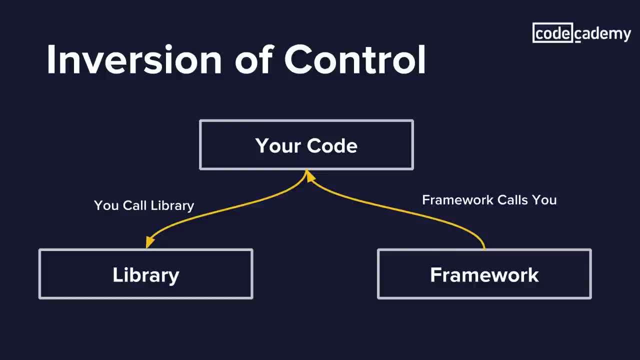 but it calls a code you plugged in as needed. Now a lot of frameworks can get quite hefty and large, like Rails for example, So for that reason, many frameworks actually end up even using libraries, But it's important to note. 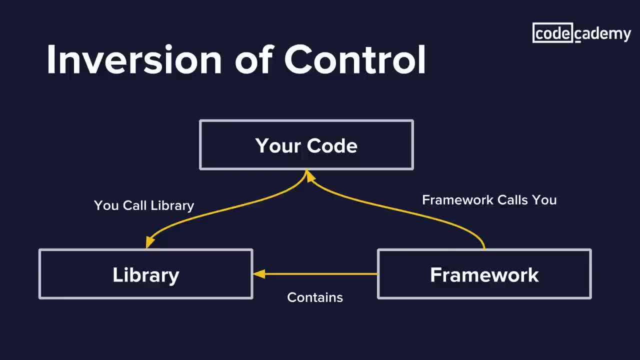 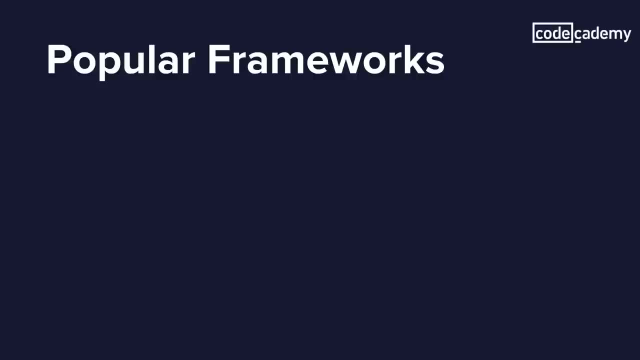 like I said in the previous slide, it's not a necessity for a framework to contain libraries. Okay, so let's go ahead and take a look at some actual popular frameworks and libraries that are used around One of the main, most popular frameworks.